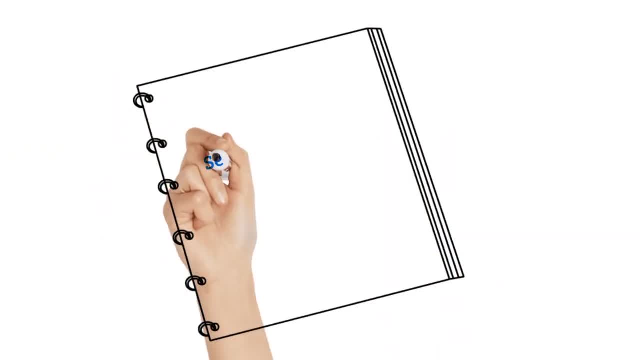 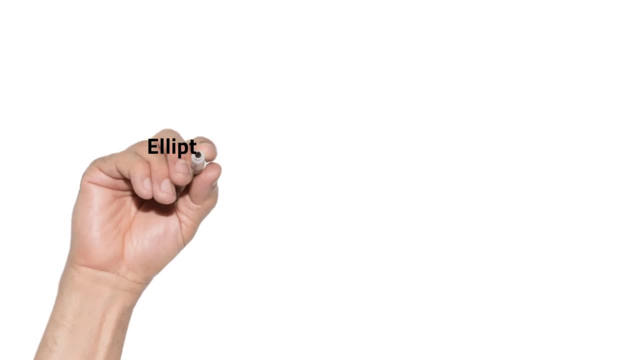 Hello all. in today's video we are going to see elliptic curve cryptography, shortened form ECC. It is a type of public key cryptography based on the algebraic structure of elliptic curves over finite field. Now let's see how it works. The basic idea. 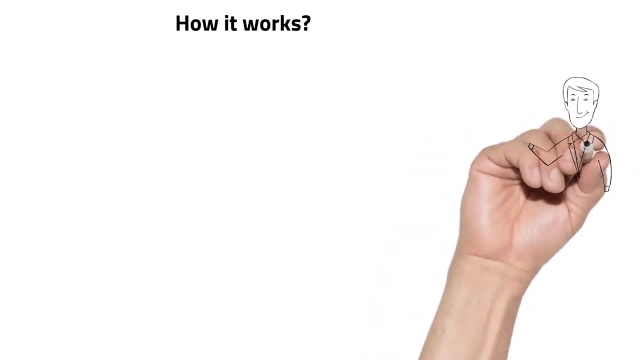 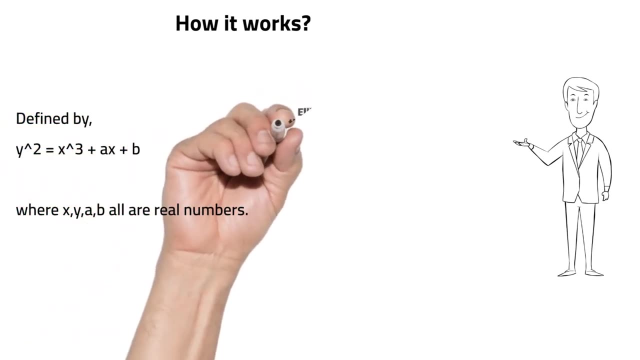 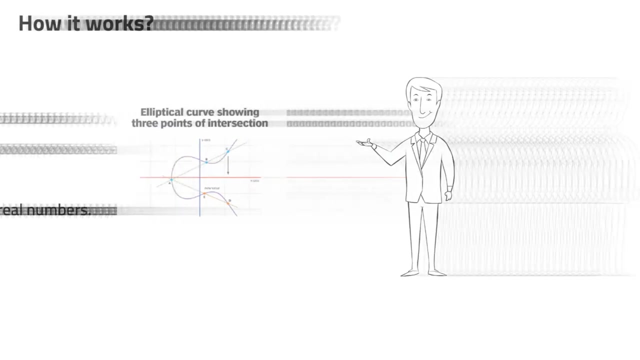 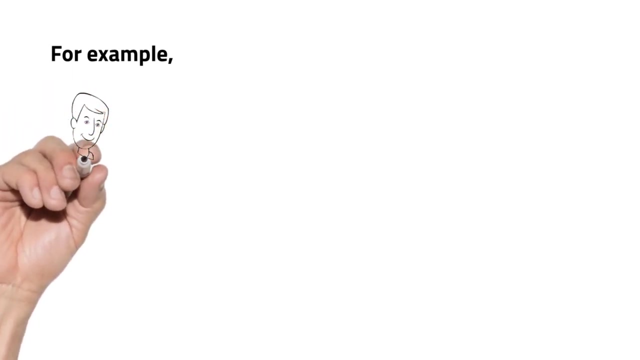 behind ECC is to use points on elliptic curve as the basis for public and private key. The curve is designed by a mathematical equation. The points on the curve are used to perform cryptographic operations. I know it is little confusing. Let me explain you with an example. Imagine the two people want to send each other secret message. They 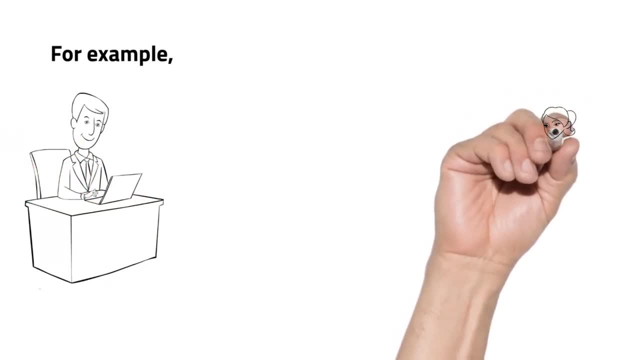 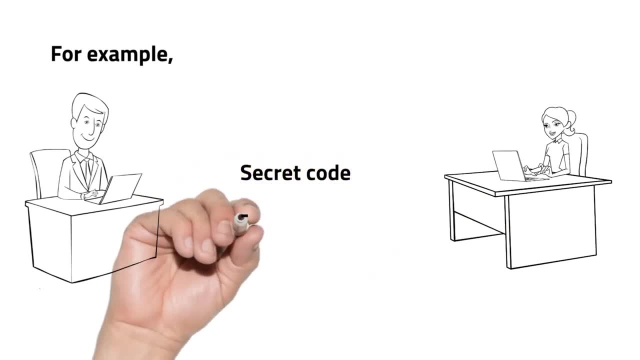 know Use it to encrypt and decrypt their message. In ECC, the secret code is replaced by mathematical equation of the elliptic curve. The point on the curve are used to perform the encryption and decryption process. Let's see how secure it is. The elliptic curve discrete algorithm. 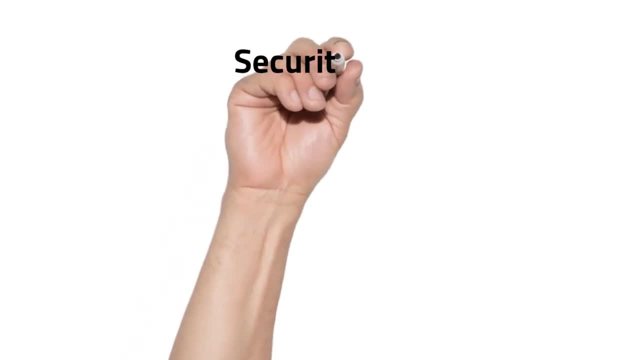 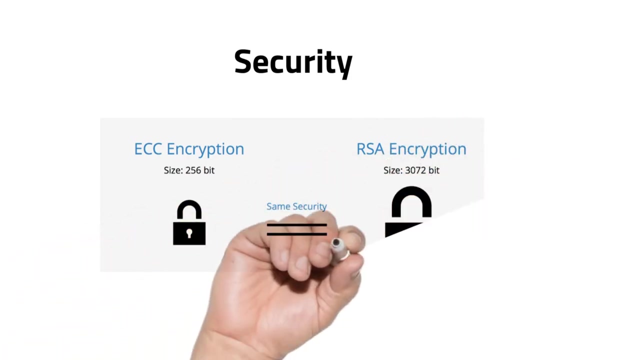 problem is the underlying security of ECC. It is believed to be computationally infeasible to solve this problem efficiently. Also, it is an advanced form of cryptography. Offers stronger security with the smaller keys, compared to other public key algorithms such as RSA. 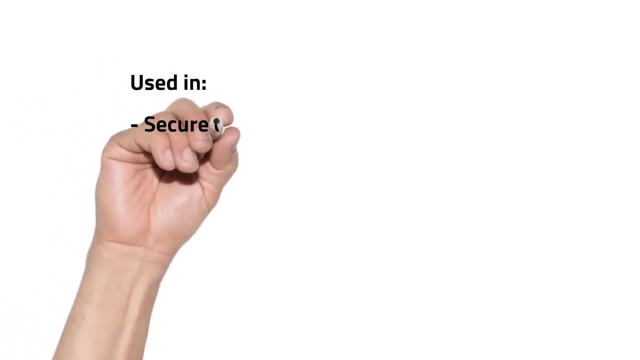 It is used in variety of application: secure communication protocol, digital signatures, key exchange. One of the main advantage of ECC is its smaller key size. Because of this, it can be used in constrained environments such as mobile device and embedded systems. Thank you for watching. 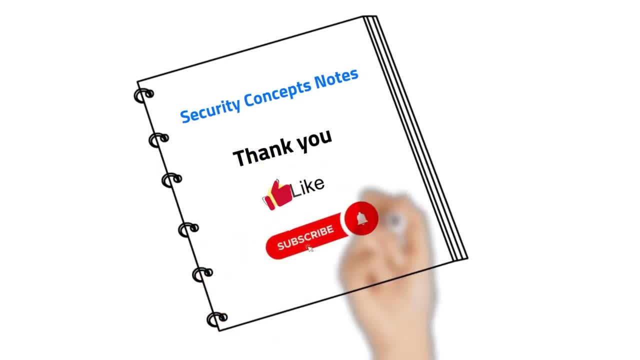 my video. Make sure to subscribe, like and don't forget to hit the notification bell. Bye.